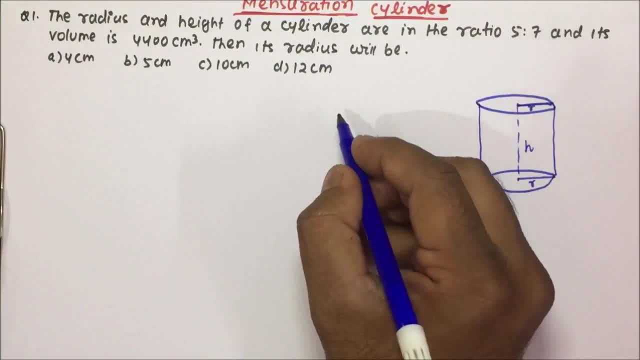 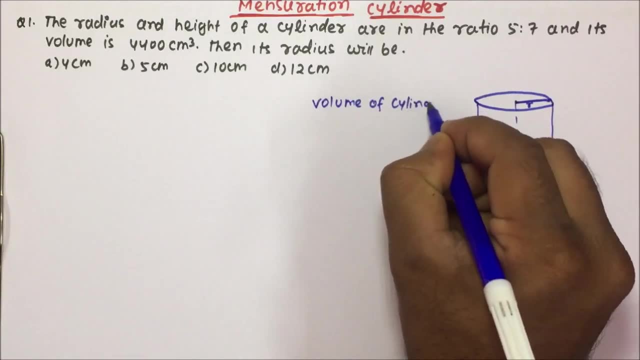 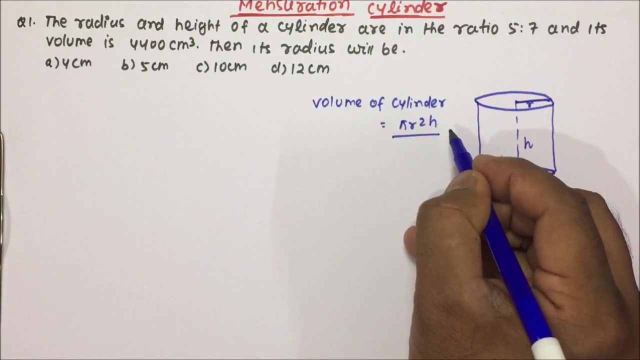 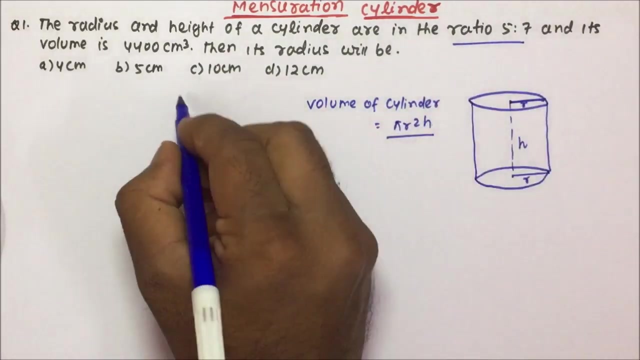 Okay now. so, friends, we will talk about the volume of the cylinder. So if we talk about the volume of the cylinder, then volume of cylinder will be equal to. so volume of the cylinder will be equal to pi r square h. Okay now, friends. so what has been given in the question? the radius and the height of a cylinder are in the ratio. five is to seven. So, friends, the radius and height of a cylinder is given in terms of ratio. 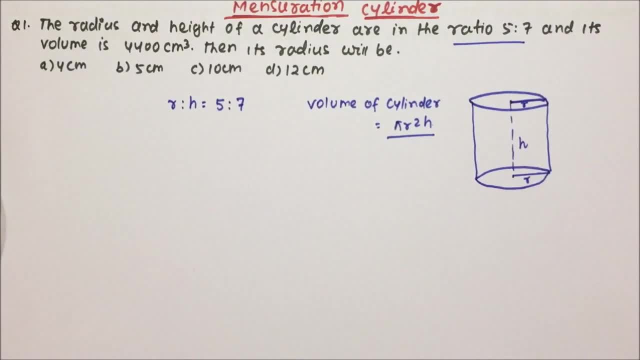 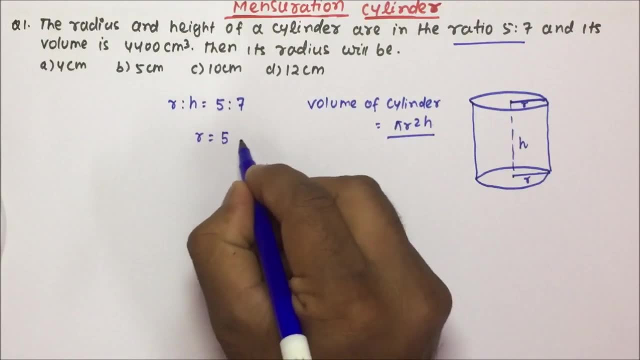 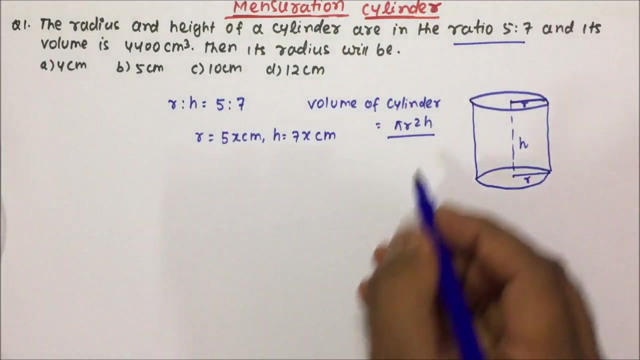 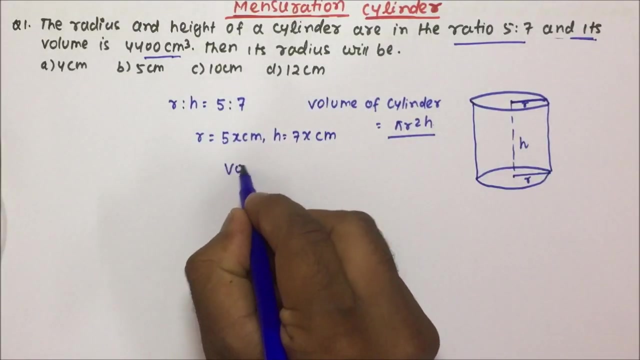 Now, friends, if any data is given in terms of ratio and if you want to write down in terms of value, then what you have to do, you have to multiply with a variable, So radius will become five x centimeter and the height will become seven x centimeter. Okay, friends, now and its volume is 4400 centimeter cube. So, friends, volume is given: 4400 centimeter cube. 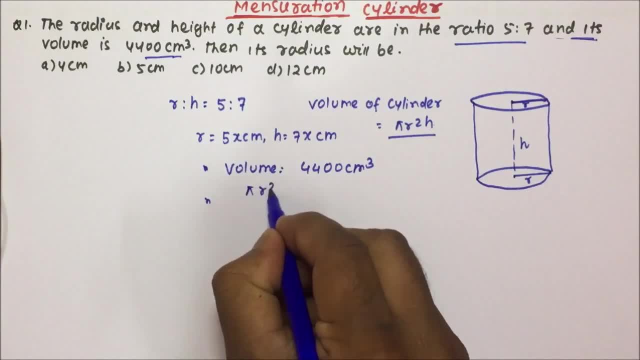 Now, and its volume is given 4400 centimeter cube. So, guys, if any data is given in terms of its volume, that is will be pi and we will have to take the radius, So volume will be pi. r square h is equals to 4400.. Now, friends, 22 by seven into radius. radius is here. you can see, friends, five x square. So five x into five x and height will be nothing. but, friend seven x is equals to 4400.. Now, friends, we have to divide this. So seven and seven will go off. And friends 22 will divide this by two times. So five and seven will go off, And seven and seven will go off. And so comes Ç Shepherd's formula이에요. 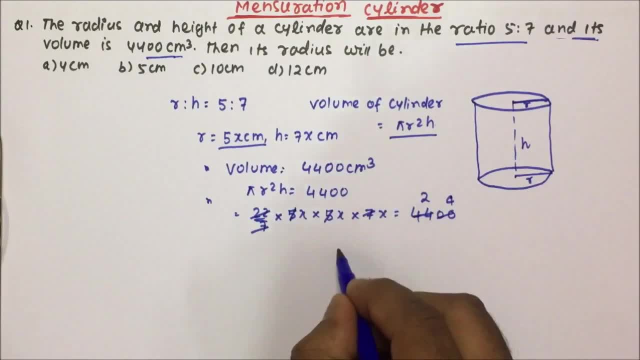 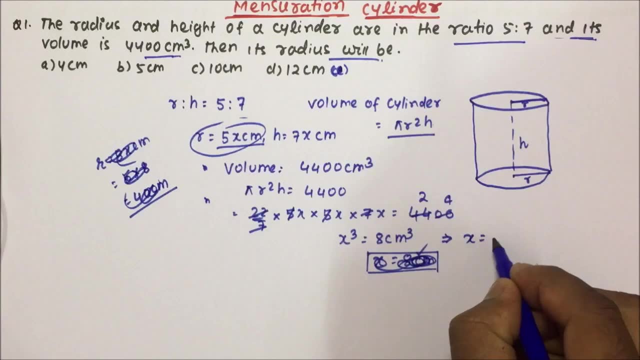 and 5 into 5 will divide this by 4 times. So, friends, x cube will be equal to 8 centimeter cube. Now, friends, the value of x will become equal to 2 centimeter Because, friends, if x, cube is equal to 8 centimeter cube, then if you calculate the cube root of 8, it will be 2.. 2 cube will be 8.. So, friends x, we got 2 centimeter. Now what has been asked? Then its radius will. 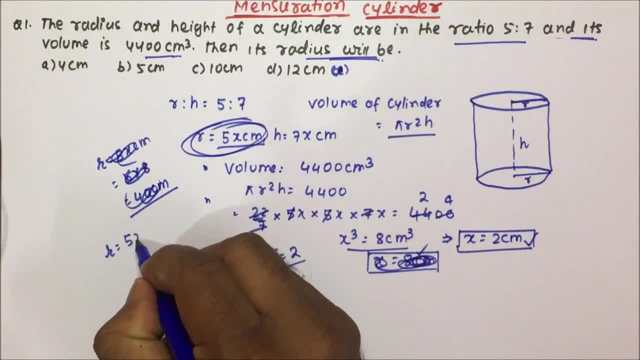 be So, friends. radius is nothing but equal to 5 x centimeter. Now the value of x which we have got from here, is 2 centimeter, So 5 into 2 centimeter, which is nothing but 10 centimeter. 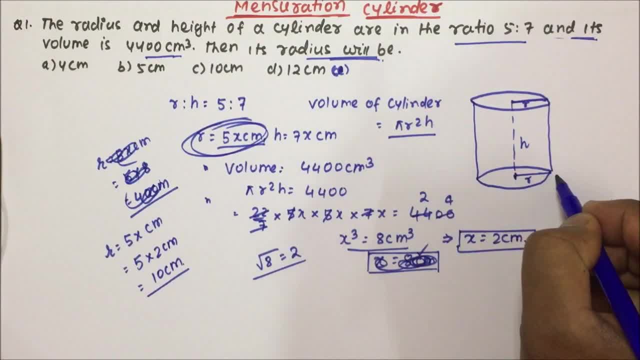 So, friends, the radius of the, the radius of the cylinder, will become equal to 10 centimeter. and you can see here, friends, option C for the question number 1 is correct. So this question we have easily solved it, friends. So only the formula you should be. 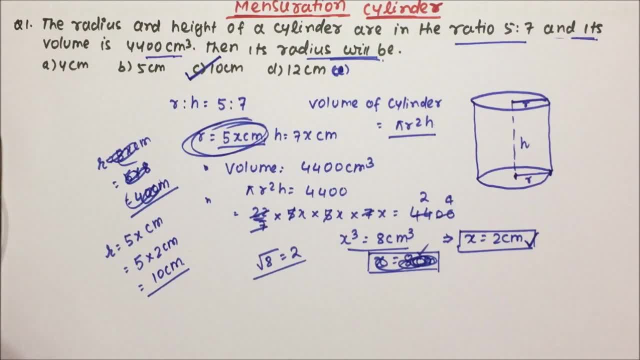 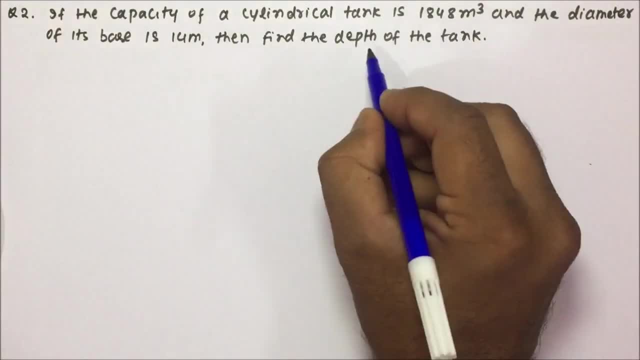 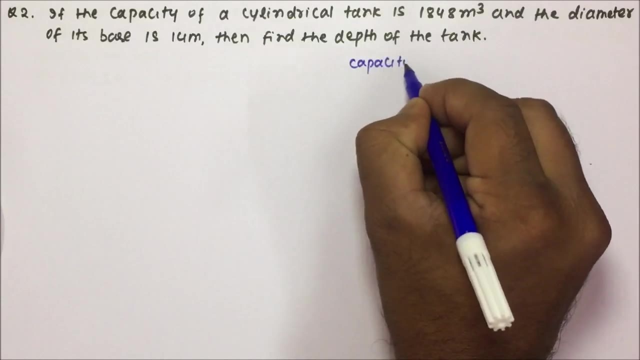 able to keep that in mind and then we will be easily able to solve with the basic concept. Now, friends, moving towards the question number 2.. Friends, question number 2. If the capacity of a cylindrical tank is 1848 meter cube, Now, friends, capacity of cylinder is nothing but. 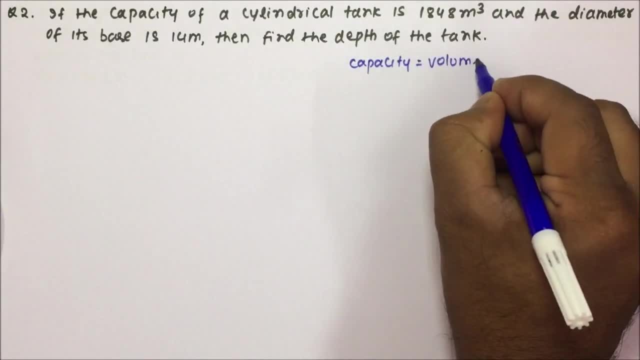 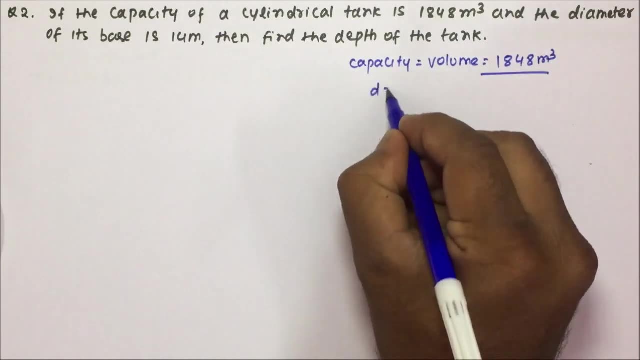 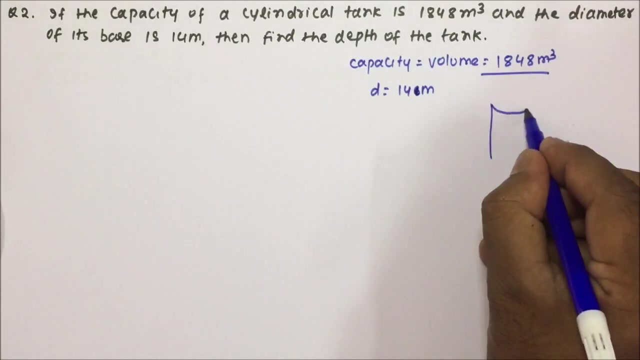 capacity of cylinder is nothing but volume has been directly given 1848 meter cube and the diameter of its base is 14 centimeter. So, friends, diameter is given 14 meter. Now, friends, if we will talk about cylinder, then cylinder look. 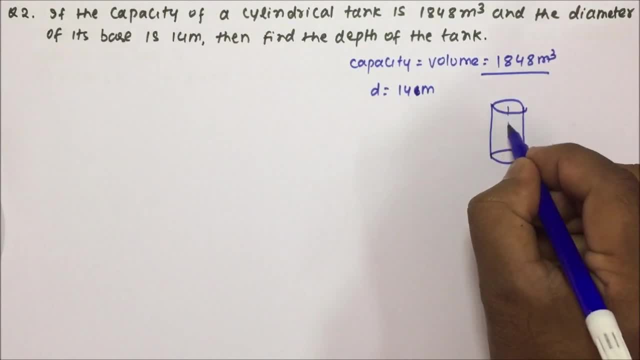 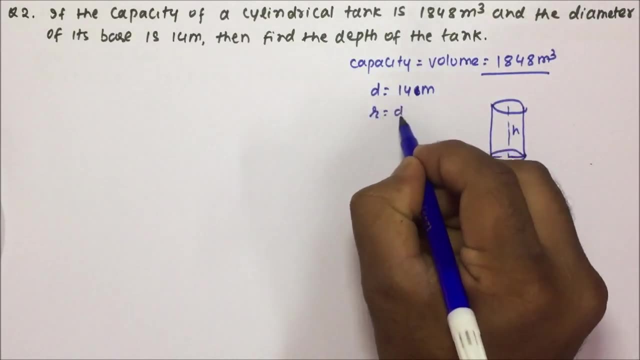 like something like that. So cylinder will look like something like that, and this will be nothing but the radius, and this will be nothing but the radius. and this is height. So diameter is given, So radius will be nothing but diameter by 2.. So 14 by 2 will be equal to. 14 by 2 will be equal to. 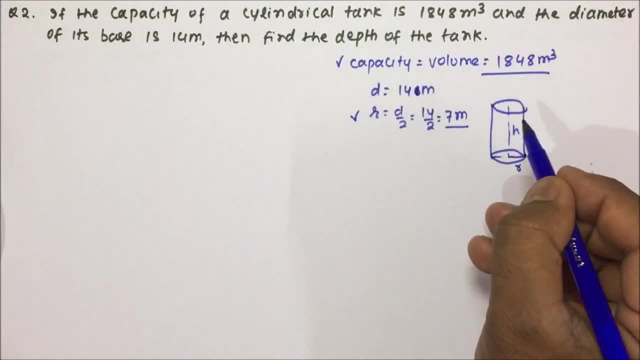 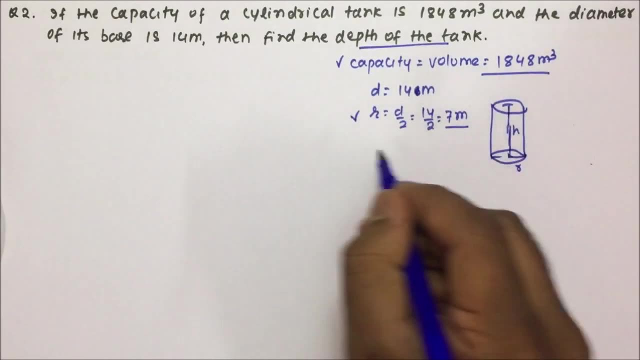 7 meter. So we have the radius and we have the capacity. that means volume of the cylinder. Then find the depth of the cylinder. So we have the radius and we have the capacity. that means volume of the cylinder, the tank. so, friend, depth of the tank means they are talking about the height. so let's, so let's. 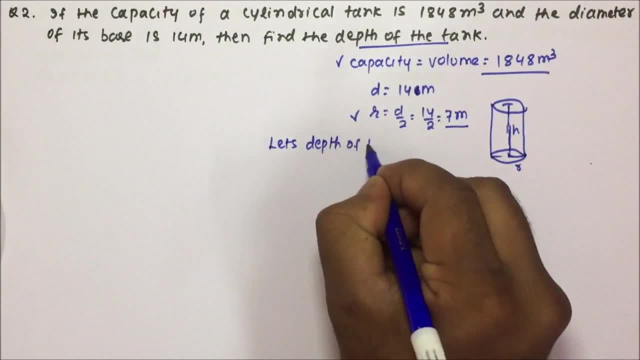 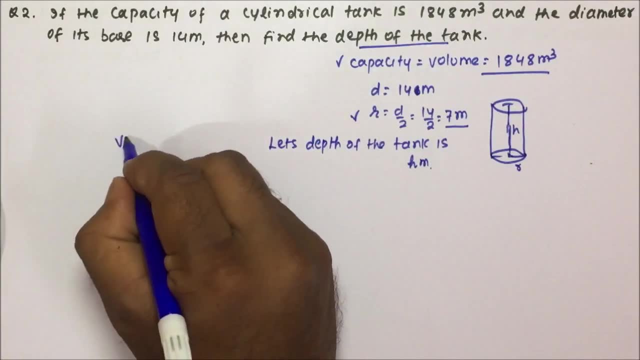 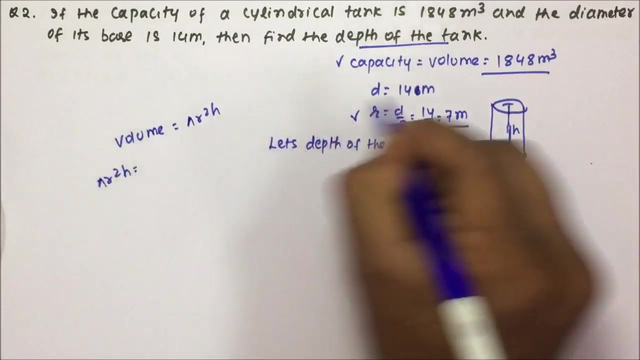 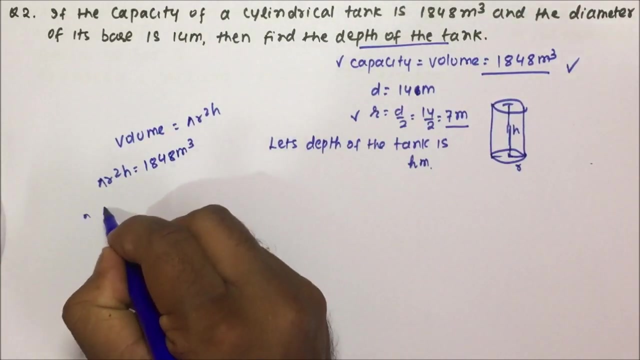 depth of the tank is let's depth of the let's depth of the tank is nothing but h meter. now, friends, volume will be equal to. so now, friends, volume will be equal to pi r square h. so pi r square h, volume is already given. 1848 meter cube. 1848 meter cube. now pi pi is nothing but friends. 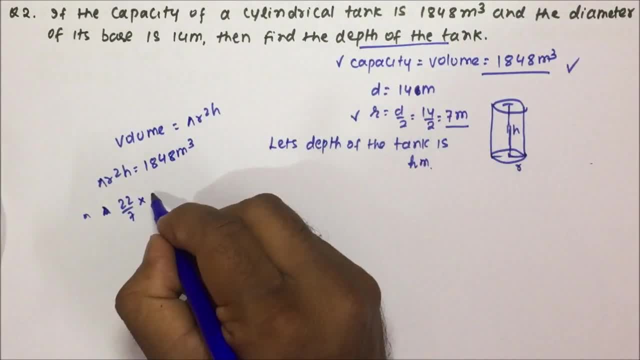 22 by 7 into. if we talk about r, so r is nothing but 7 into 7 and h. we have to calculate 1848. okay, friends, now 7 and 7 will get cancelled, so h will be equal to 1848 divided by 22 into 7. 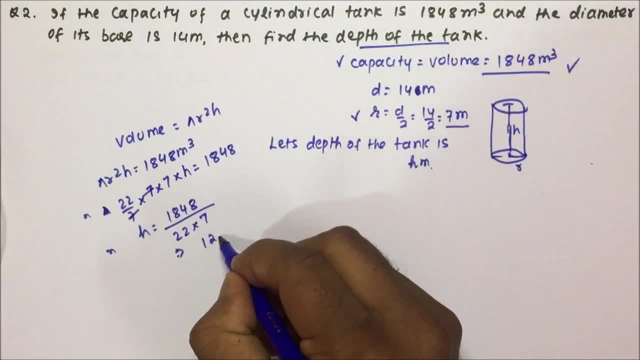 and now, friends, if we try it divide it, it will get divided by. it will get divided by 12 times, so 12 meter. so 12 meter will be the 12 meter will be the depth of the tank. so, friends, for this question the answer will be 12 meter, and it was a very good question. so today we did few basic question based on the. 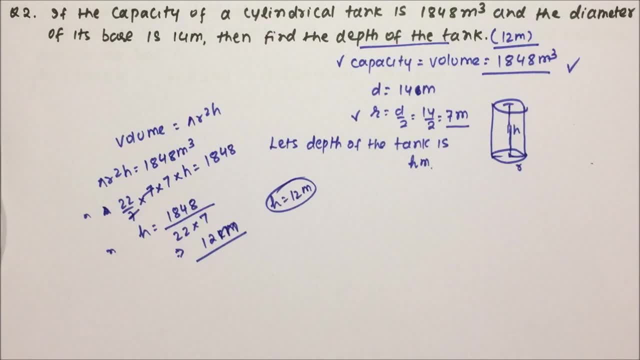 cylinder and that kind of question, friend, will definitely be asked in your exam because many of the exam needs direct formula based question. so, friends, thanks a lot for watching the video.